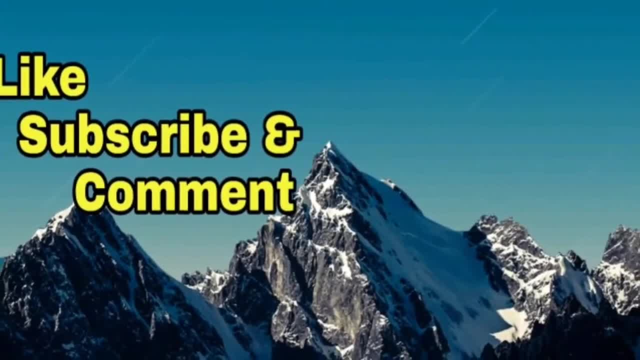 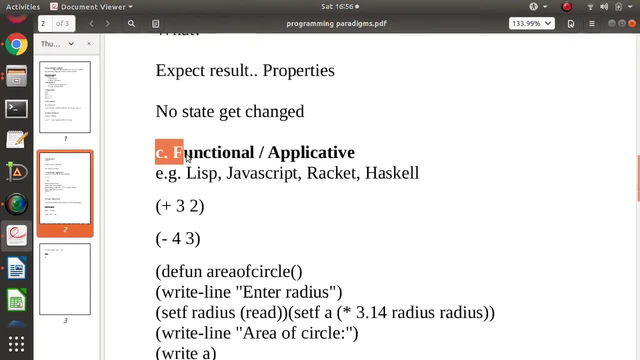 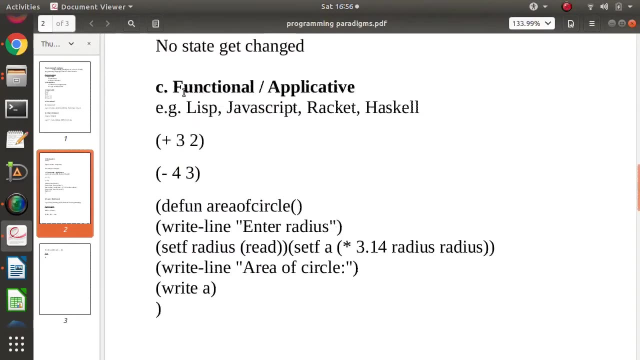 Now in declarative programming paradigm, again, there are two types, so functional, and another is logic, So functional programming paradigm. examples of functional programming paradigms are Lisp, JavaScript, Racket, Haskell. All these programming languages follow functional programming paradigm. So what is functional programming paradigm Here? all statements. 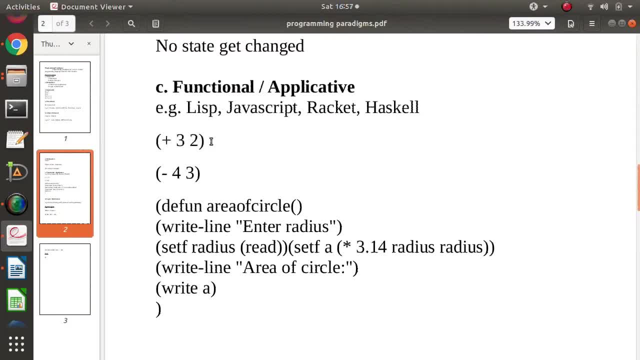 are written as a functional call, function call, For example. see: these are the statements I have written from the Lisp programming language. Now look at this: this is addition, So for addition. again we are calling a function plus, So here addition plus is a function. 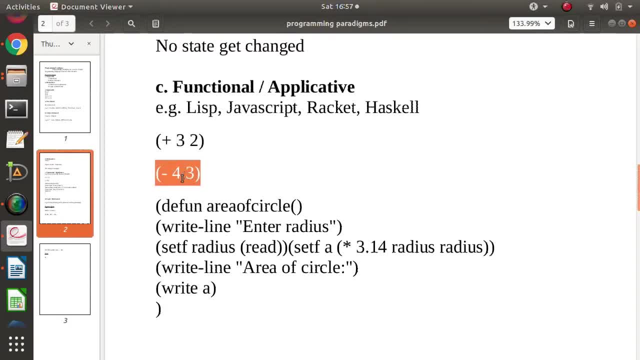 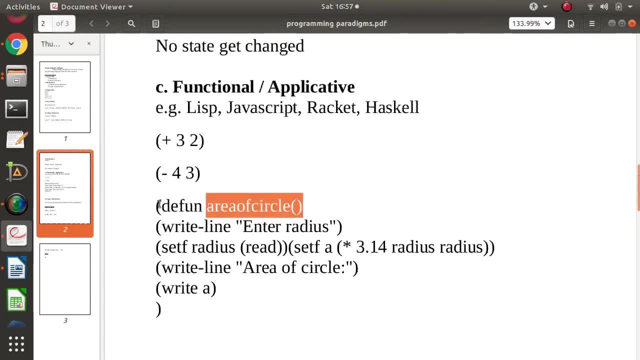 Even to define a function, we use one function. So define is a function which is used to define another function, area of circle. So example I have taken here: area of circle. So to define a function, again we require a function. So these are the statements in 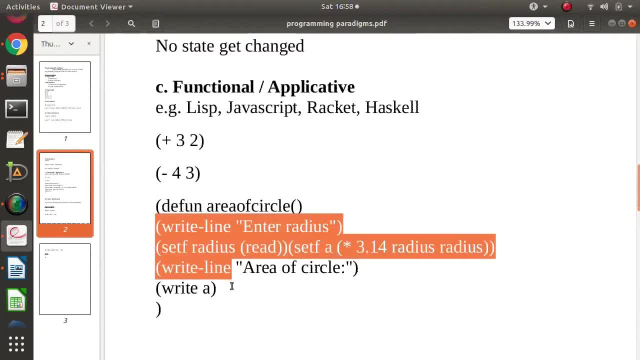 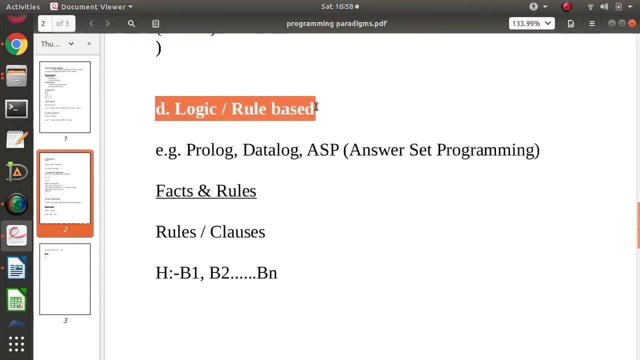 this area of circle function. So all these are a function call. So write line set in right, line right: all these are the function calls. So in functional programming paradigms all statements are the function calls. Now we'll see another programming paradigm, that is logic or rule based programming paradigm. 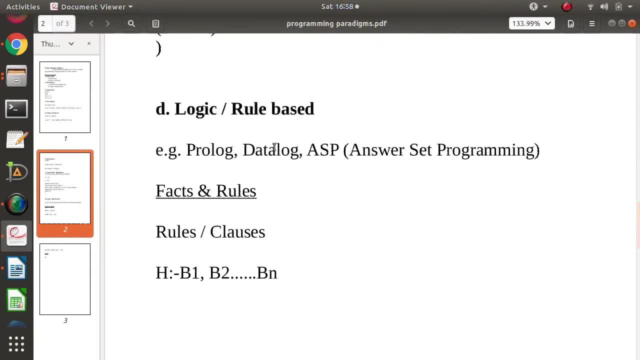 So again, it is the type of declarative programming paradigm. Examples of logic or rule based programming paradigm are: Prolog, Datalog, ASP. ASP means answer, set programming. Here every statement is facts and rules. All statements in logic or rule based programming paradigm are the facts and rules.